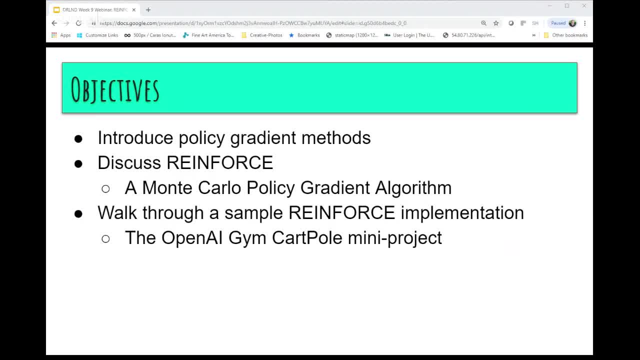 Reinforce. It's a Monte Carlo policy grading algorithm And since it's Monte Carlo, we'll see that it requires you to actually do an entire episode in order to do the learning process, the training process, So it's not a temporal difference method that you can. 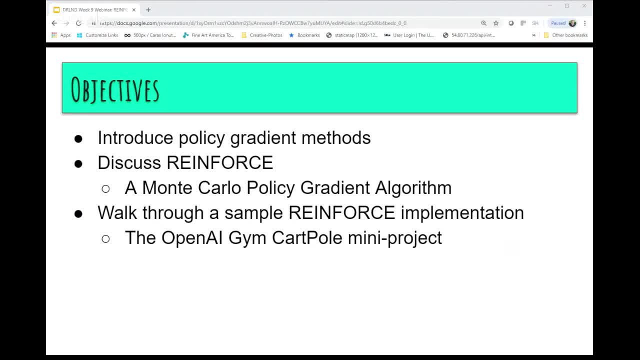 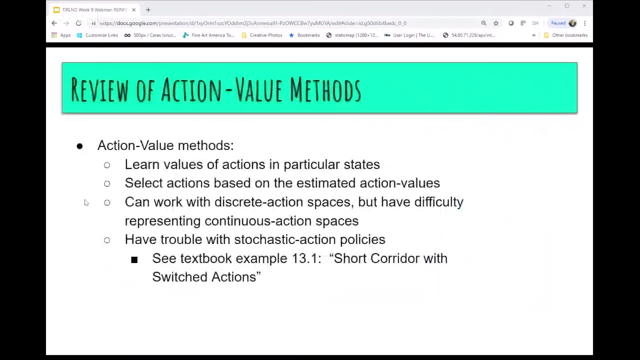 do step by step. It rather requires you to actually go through and complete an entire episode before you apply all the learning throughout. Now we'll walk through a sample of implementation of reinforce in the OpenAI AI Gems CartPoll mini project. So let's start with some general theory about gradient methods, policy gradient methods. 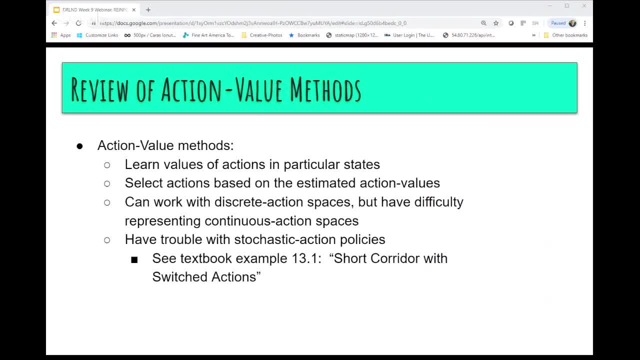 Before we do that, though, I probably should mention that, up to this point in the course, most of the work that you've done and that we've talked about have been associated with action value methods, So it's worth probably reviewing what those are to contrast them with the policy gradient. 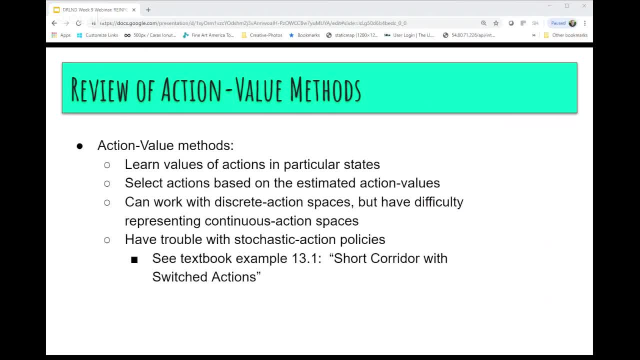 methods. So action value methods. they learn values of actions in particular states And then once those values of those different actions are determined in the state, then the approach is to select the action And when you're in a particular state that most optimizes the reward or the return for. 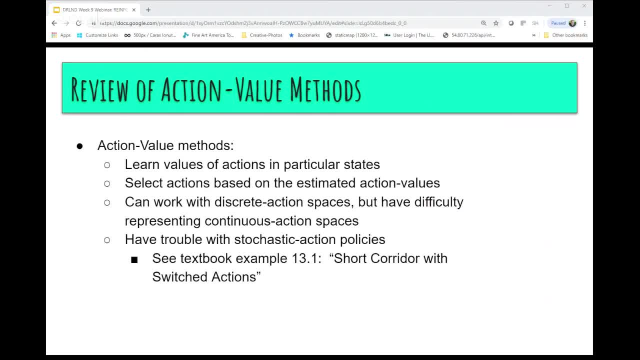 that particular state. they can work really well with discrete action spaces, But since you're really selecting a particular action based on those specific predetermined or calculated action values, they don't really work very well with continuous action spaces. So one thing we'll find out with these policy gradient methods are that they really do work. 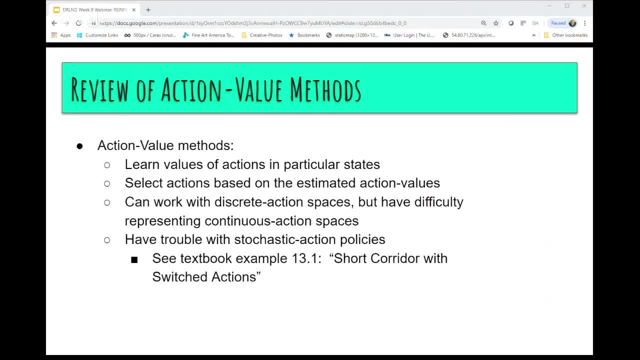 well with the continuous action spaces. So if you have a problem where you have to choose continuous-type actions rather than discrete actions, policy gradient methods is a way to go. The other thing is that action value methods they sometimes or often have trouble with. 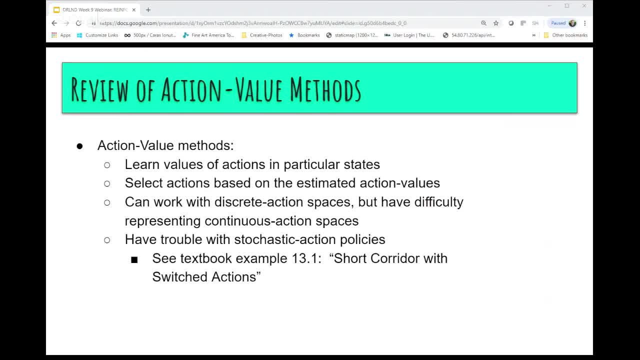 stochastic action policies. There's an example in the textbook 13.1, called a short corridor with switched actions, And in that particular example it's a pretty simple example, But you basically have to. I tried to get to a terminal state that gives a good reward. 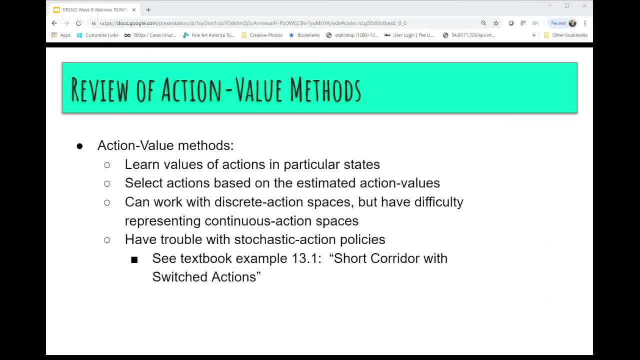 But whereas normally you go right when you select the right action in most of these states, in one of the states when you select right, the environment actually has you go left And if you select left it actually switches that and goes right. 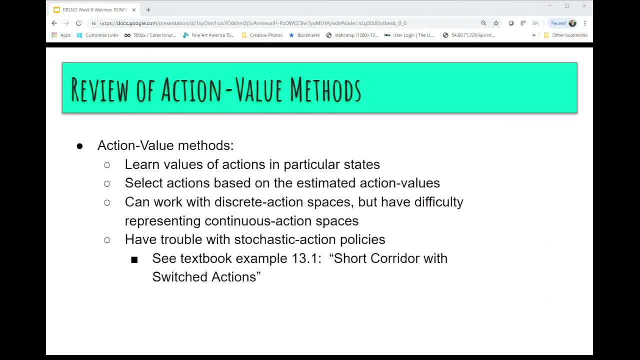 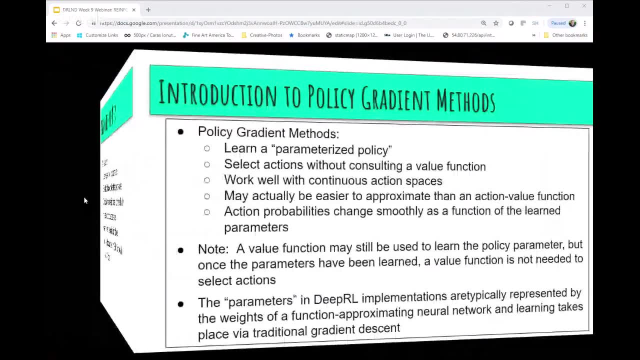 And you can look through that example and see how an action value method would have a very difficult time solving those types of problems. So with that quick overview of the action value method, I'm going to turn it over to the next speaker. Thank you. 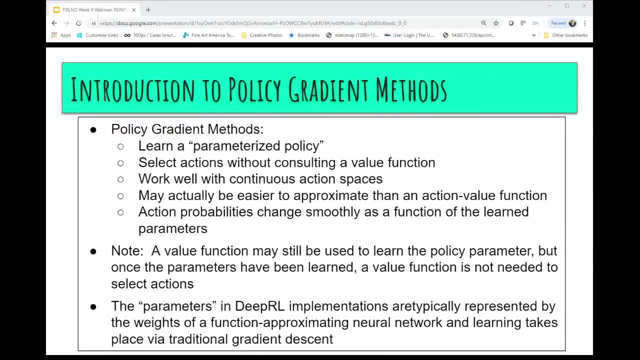 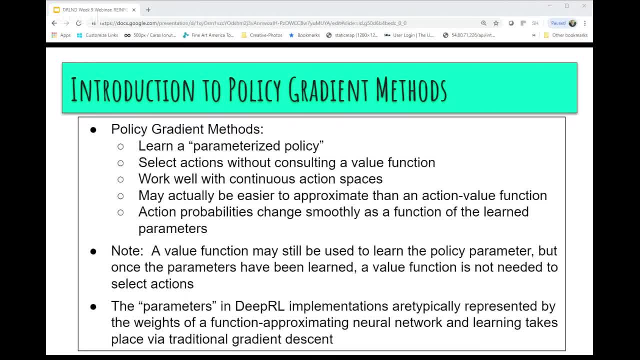 And we'll find out here in a second that the parameters that we use actually are the weights of a neural network, And all the combinations of all the weights become that parameter, uh, theta, uh, that determines, uh, how, what, what policy is being employed? so you could think of: 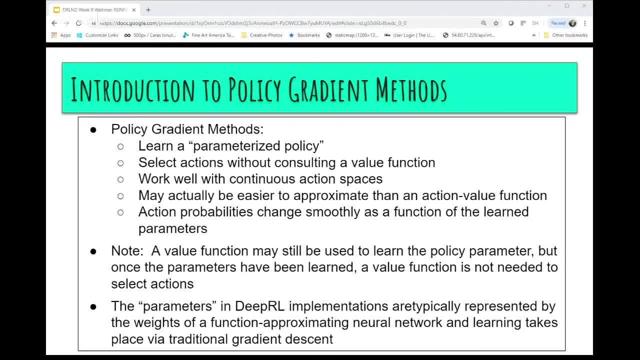 uh, you know like an optimal policy and a previous method might be to, in each particular state, uh select the optimal action uh from the calculated action values that if you're using one of those earlier methods, in this case the policy is actually represented by those weights of a. 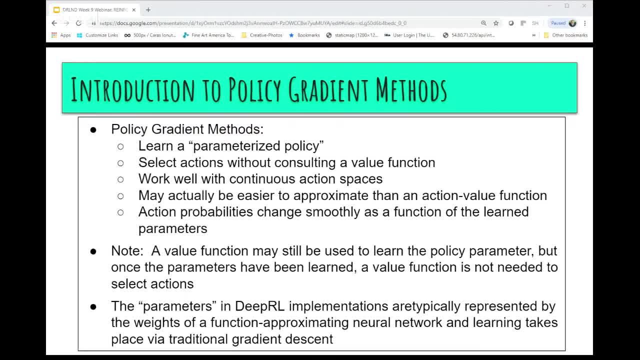 neural network. so, given a state that you're in, those neural network, weights determine the policy and they're used to then, through a form of propagation, select an action from that input state and in the parameterized policy. so a unique feature of these policy gradient methods is that 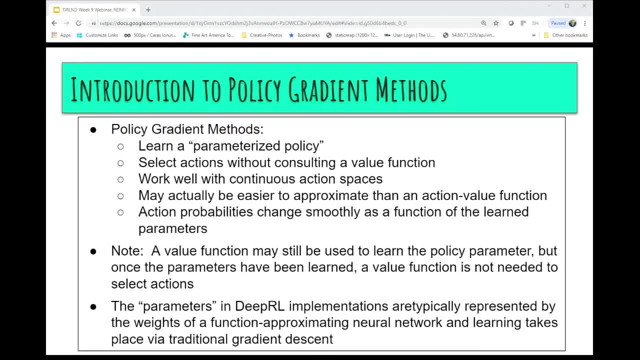 they can select actions without consulting a value function, so you don't have to calculate value functions in the process selecting actions. but you will also see that we will use those value functions in order to train the network. but once it's trained it's no longer necessary to to 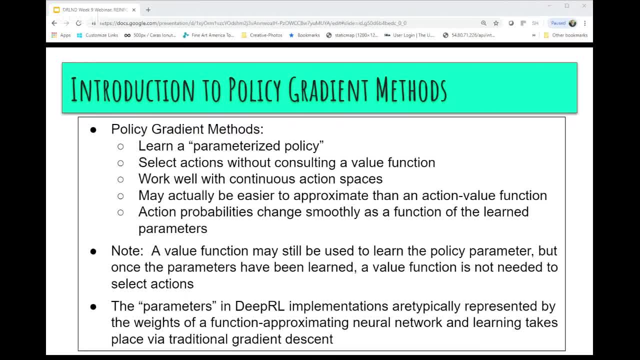 calculate value functions, the policies embedded in the weights of that neural network and you just do a forward propagation step and you get the action based on the state inputs. other interesting advantage of policy gradient methods i mentioned earlier is that they work well with continuous action: spaces, spaces. so we can see that you know the output actions that you would get. 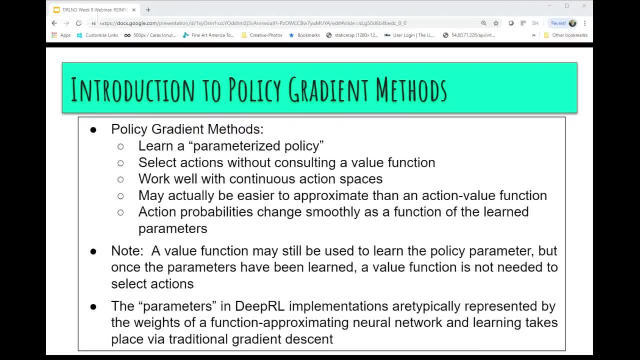 in the final layer of a neural network can be continuous values, and so those actions that you select with this method also work well with those continuous action spaces. i'll also find that it actually could be easier to approximate a policy gradient or policy set of parameters than it is to approximate the action value functions that 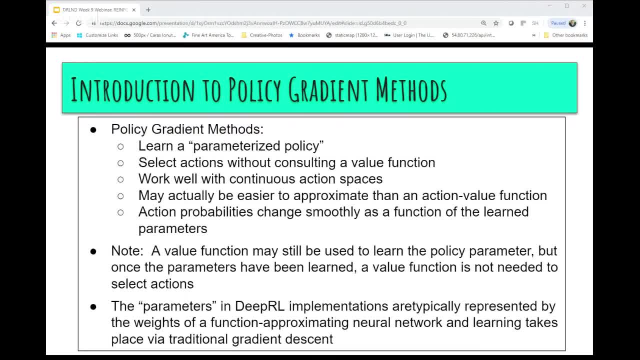 we have been using previously, and the final unique feature of these algorithms- that's very advantageous- is that these action probabilities change smoothly as a function of the learned parameters. so those learned parameters are the weights, as i said, of a neural network. we'll see in a second and we're going to talk a little bit more about that in a 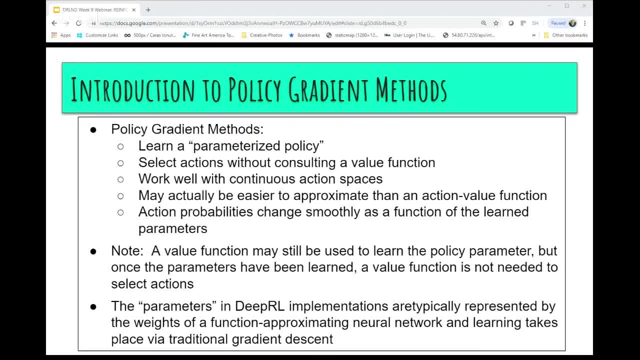 moment. um, as those uh, as those weights change smoothly in small increments, the actions also. probably the actions also change. that's not really true in an action value method, because uh, a slight change in, in, in, uh, a value, uh, would have maybe a, perhaps a a large change in the action that you would choose. so they expect you know. 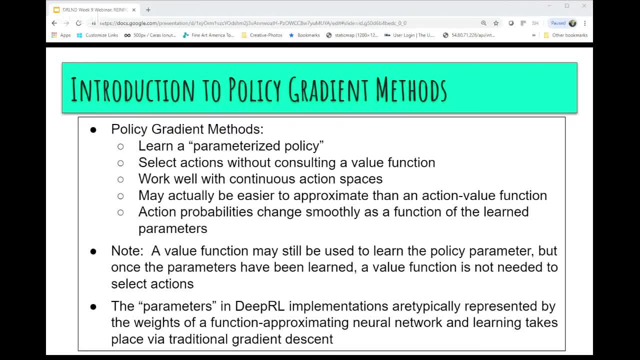 you see that a lot in discrete kind of action spaces in general. so, as i mentioned, uh, we might be calculating value functions. we will be calculating value functions while you're learning the policy parameters, but once you've learned those policy parameters, once the weights have been established, 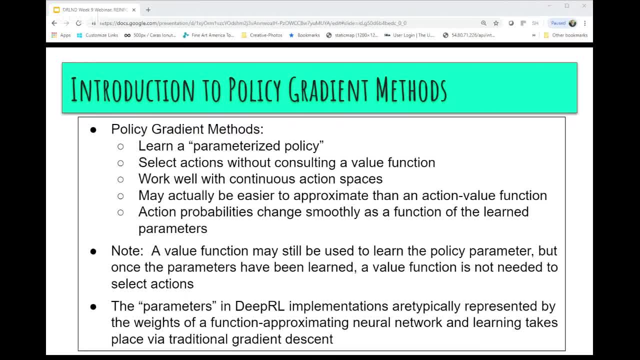 in the policy function, then the value function is no longer needed and, as i've been referencing here for a bit, the, the parameters that we're talking about here, in a deep reinforcement learning, become the weights of a function approximating neural network. so again, we talked a few webinars. 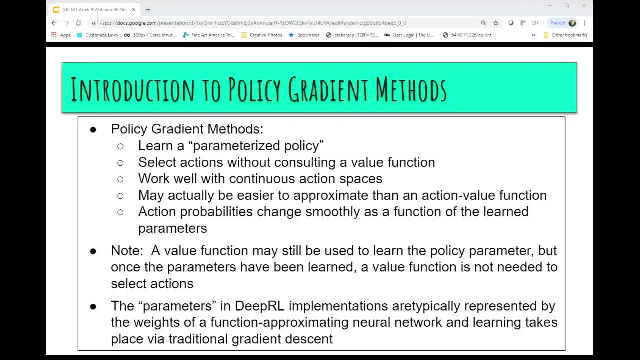 about uh, that, uh, we're talking about uh, that we're talking about uh, a lot about uh, the data management and uh, and the other thing is that uh, neural networks are excellent universal function approximators and here they're being used uh, in the same way, and the function of 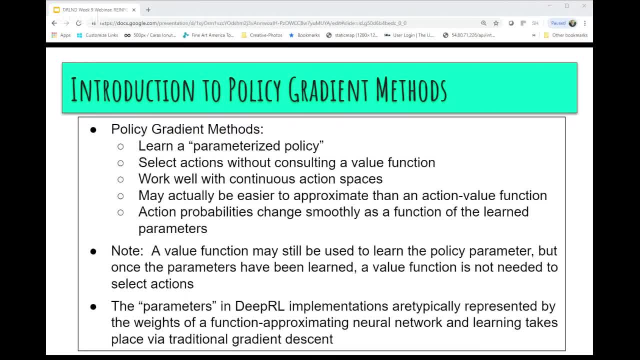 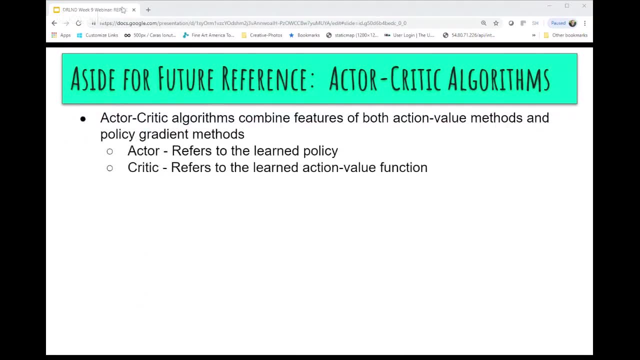 approximating is the policy function. so, um, we use traditional uh gradient descent to train these types of networks and it's- uh, you know, the theory behind it is very strong and, uh, it works very well here. this reinforced algorithm we're going to talk about is the first introduction to a policy gradient algorithm. 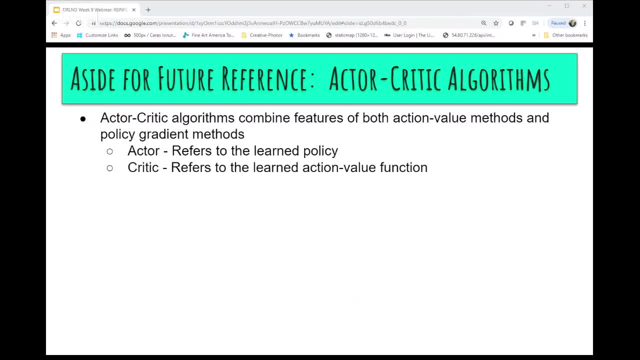 It's a very simple algorithm. we'll see And in reality in most real-world problems you probably don't use reinforced too much. Sometimes it's used as a baseline to compare other algorithms against. But you'll find in subsequent lectures and the final two, 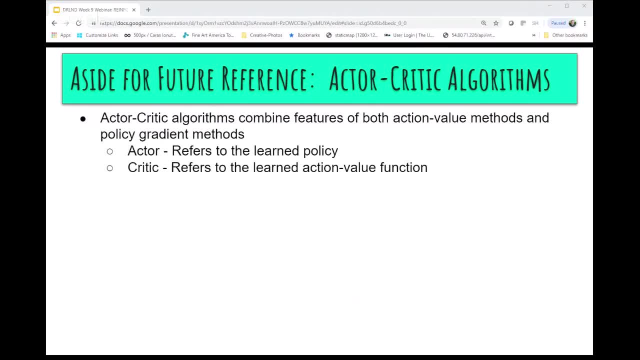 projects of the course, you're probably going to end up using a state-of-the-art type of algorithm called an actor-critic algorithm, And there's many variations of these actor-critic algorithms, But in real problems you'll be using those. 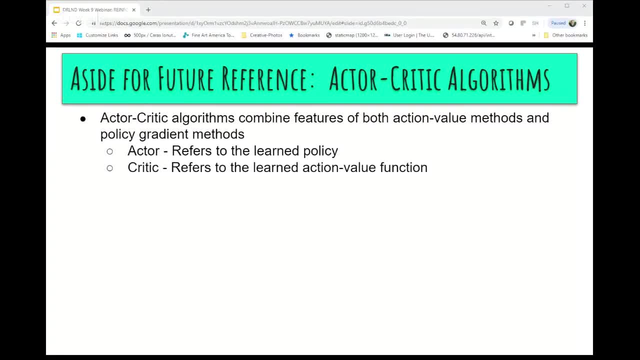 And the actor-critic problems actually have two parts: an actor and a critic. And again, this is just a quick aside and introduction, But the actor part of it. it actually is a gradient, a policy gradient method. It learns the policy and selects. 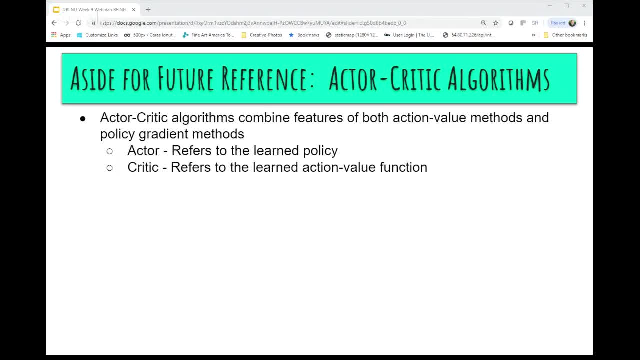 based on the inputs and that learned policy parameters, it selects an action to take. So that's the actor And then the critic is used as a traditional action value function And it's used to sort of evaluate the actor and provide some feedback that helps improve the actions. 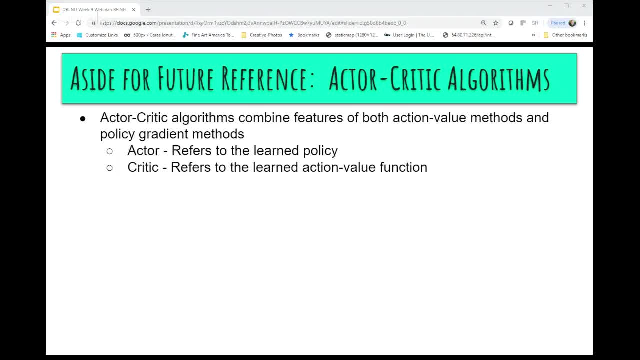 that you select. So those actor-critic algorithms, as I said, are more state-of-the-art And those are the algorithms that you actually use. But it's good to understand a simple algorithm like the reinforced algorithm to get a better understanding of these actor-critics when you get to that point. 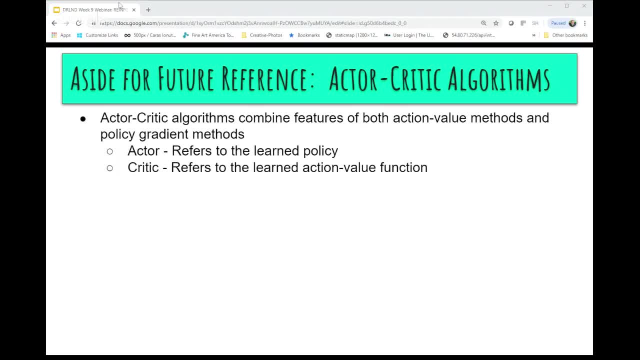 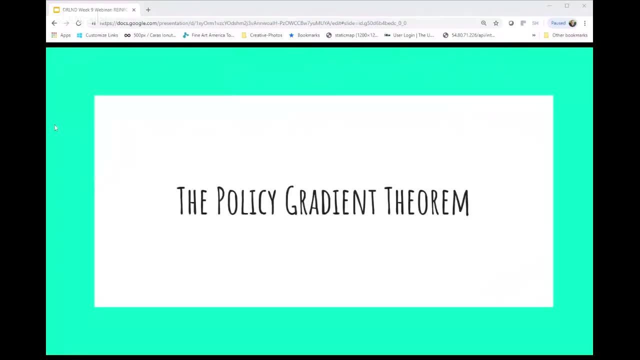 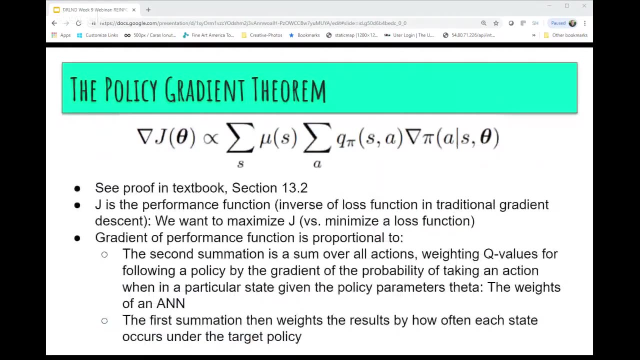 here in the course, And that's what we're going to do in the next week or two. OK, I'm not going to go into too much detail on the policy gradient theorem, but I will introduce it to you here. This is the statement of the theorem: the policy gradient. 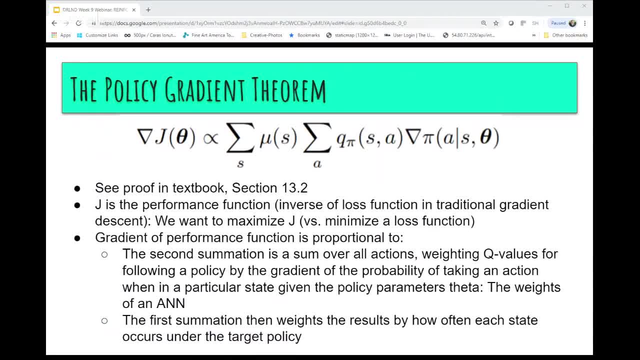 theorem. There's a proof in the textbook. It's a single-page proof And you can follow that along in section 13.2 of the textbook if you'd like to see the details of that. But I'd just like to talk a little bit about this theorem. 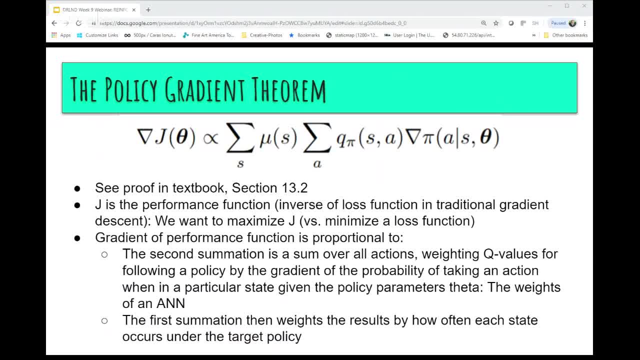 and explain sort of how it operates and sort of intuitively how it probably makes sense that this type of an approach would work. So the first thing is on the left side there is something called J, If you're used to developing a loss function for a neural network. 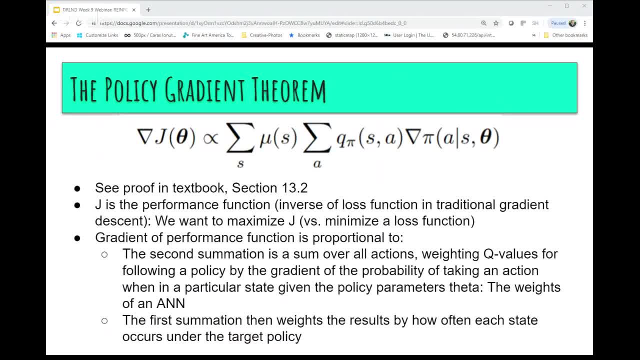 to do gradient descent on. this is sort of the opposite of a loss function. It's a performance function. So it's the inverse of a loss. It's a gradient descent. In a traditional gradient descent you'd want to minimize the loss. 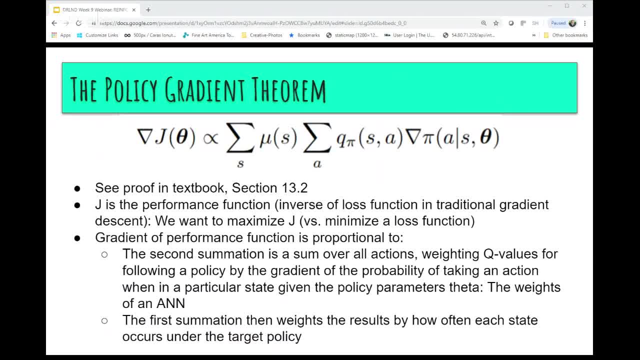 Here you want to maximize the performance, You want to maximize J. So this J function is a function of the parameters of the neural network, theta. Those are, as you'll see in a bit, for us in deep RL, those data values are just the weights. 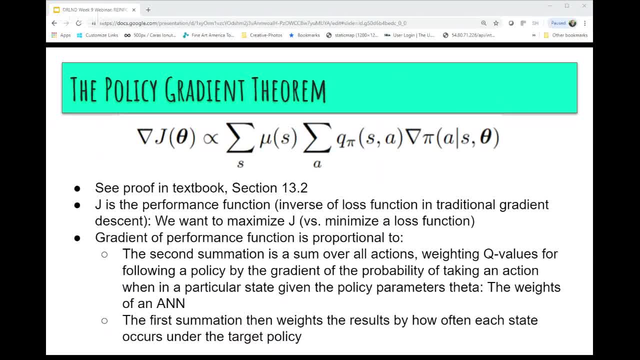 of the universal function approximating neural network that we're using, So that performance function is proportional to a couple things. The two things on the right that you see, there are the proportionality values. Let's talk about the second half of that first of all. 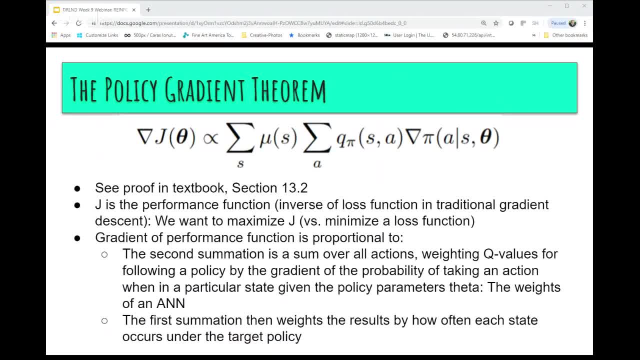 That second summation. as you can see, it's over all actions, So you sum over all actions. You weight the Q values that you get following that policy for a Q value and a state action pair by the gradient of the probability of taking that particular action when you're in the given state. 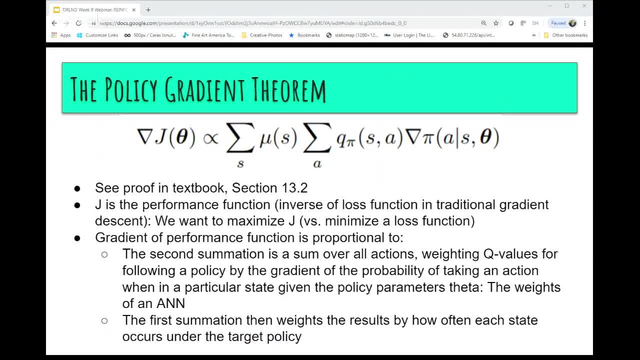 Given the current policy parameters data, which is again the weights of the neural network. So that kind of makes sense. You're going to weight the values that you get by the probability of taking that action in that state. So that seems to make sense. 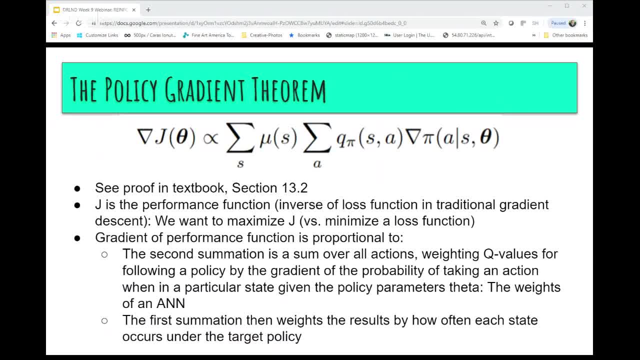 And then the first summation then weights those results by how often each state occurs under the target policy. So that essentially is the policy gradient theorem, And we're now going to be applying that in this algorithm called Reinforce. So the Reinforce algorithm. 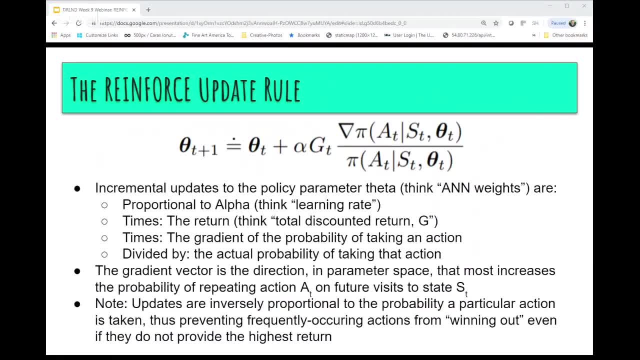 This, as I mentioned earlier, is a Monte Carlo. I don't actually have that on the slide here, but it's a Monte Carlo technique. But we are going to update a particular state, a particular set of weights. Sorry, I was on a state. 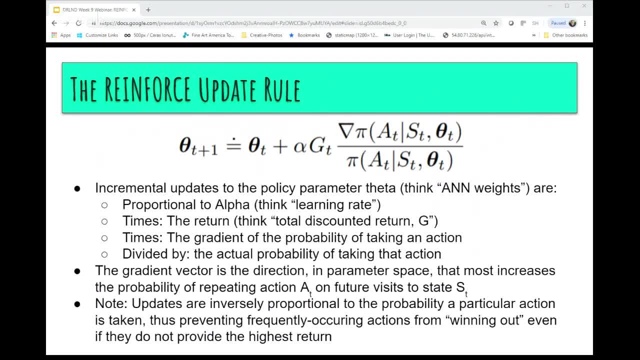 A particular set of weights are going to be updated with this formula. So the new values for the weights is going to be the old values of the weights plus this term on the right of the equation. you see here, And there's three or four different parts. 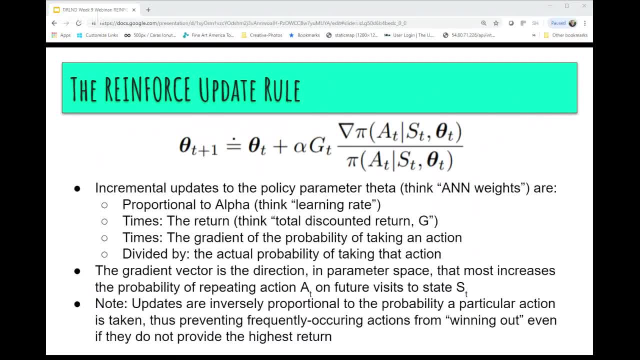 to this equation. The first part is alpha. You can think of that as a traditional learning rate in a gradient descent type of learning, neural network, backpropagation learning method. You're going to take that learning rate times the total return, total discounted return G And that's going to be times the. 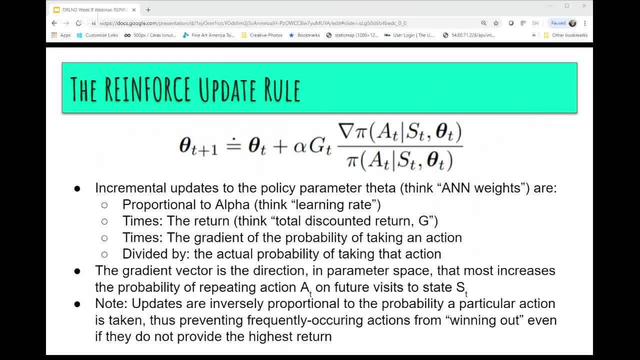 gradient of the probability of taking a particular action divided by the actual probability of taking that action. Now, the interesting thing about this is is the third bullet I have here, And that is that the updates, as you can see are, are proportional to the gradient, but they're. 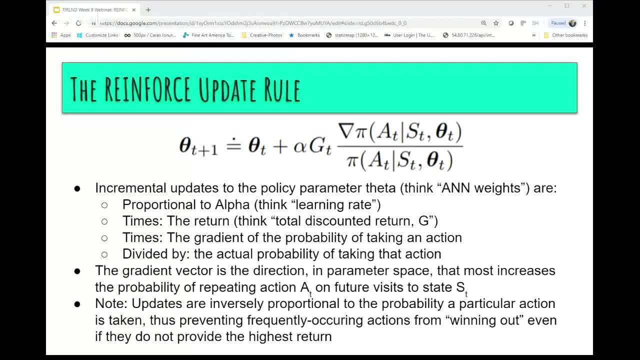 inversely proportional from the probability of particular actions taken. And this has some kind of intuitive appeal because it prevents really frequently occurring actions from dominating the results, even if they don't provide the highest return. So dividing by that that probability of occurrence kind of mitigates that particular feature and 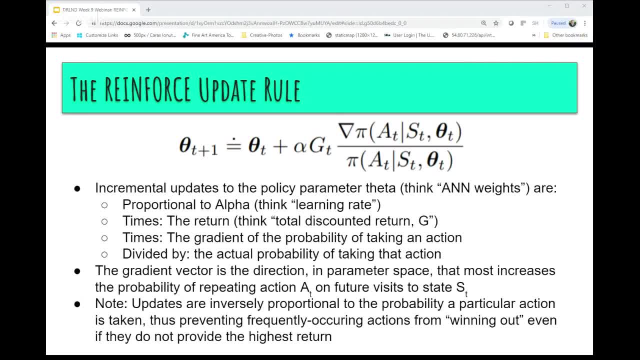 then sort of optimizes the results for the actual returns that provide the best reward, best total reward. And remember the gradient: it's a vector And the gradient is the direction and parameter space, which, again, parameter space for us, is the weights of the neural. 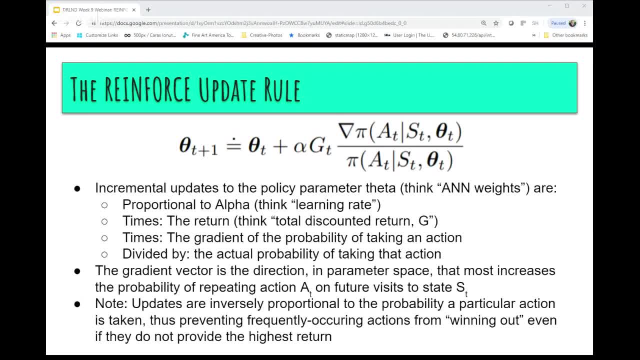 network, the space that is determined by those weights, The gradient, is the direction in that space that most increases the probability of repeating a particular action on future visits to that same state that we're that we're evaluating here. So, as you can see that that's intuitively, it seems to. 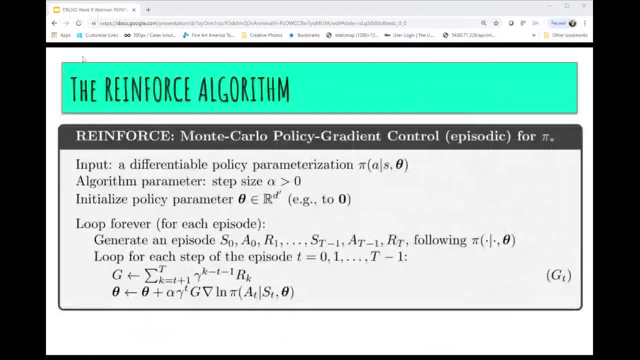 kind of make sense. It's pretty simple update rule. So let's look here at the actual algorithm, And this is the Monte Carlo policy gradient algorithm, as stated in our textbook, should have put the page number something on here, But if you look up the reinforce algorithm you'll see this. this: 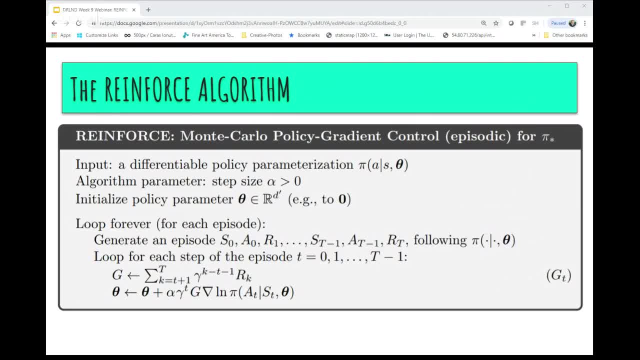 pseudocode for how it's implemented. As you can see, it's a pretty simple algorithm. You input, basically, a differentiable policy, pi that determines a direction given, a state, and the- the parameters of the neural network in this case. So it's going to do this, this policy. 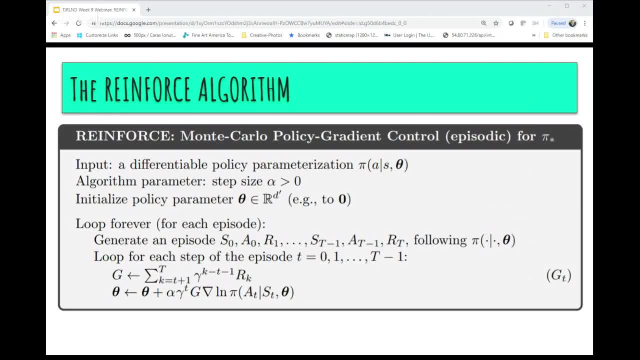 says, if you're in this state and we have this set of weights in the neural network, you can run through a forward propagation step and determine what the actions should be. Another input to this algorithm, as we've mentioned in the previous slide, is the step size alpha. that's kind of the 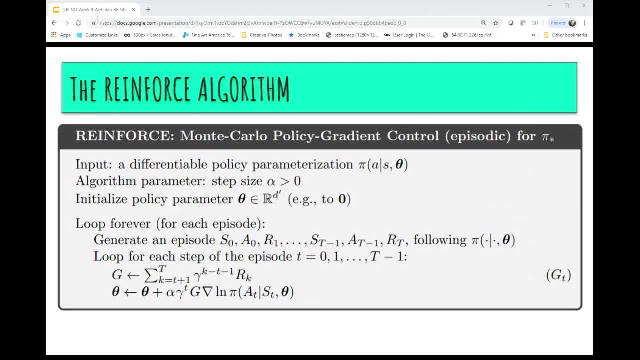 learning rate parameter And the first thing you do is initialize all the policy parameters data to some value. Sometimes this is set. all the weights will be set to zero. There's other research that's been shown to say that zero is probably not perhaps the 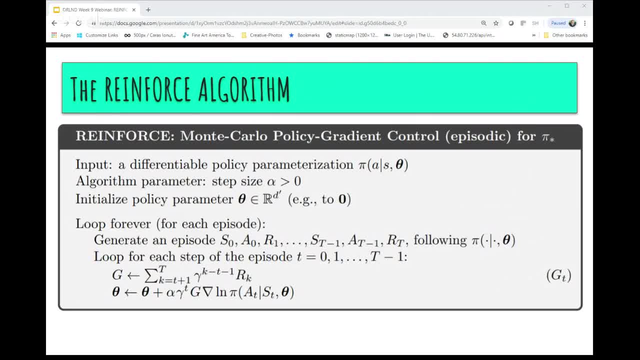 best value to use, And there's a lot of different research papers on how to choose a better value for theta. But in essence, you need to choose some value as the initialized values for all the weights of the neural network. Once you do that, then you 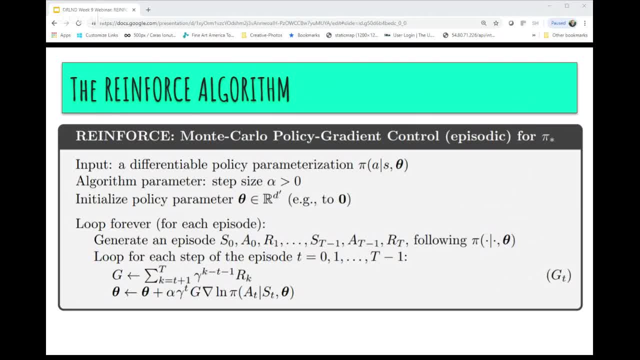 basically go into a loop. You go through this loop once for each episode. As I mentioned, it's Monte Carlo technique, So we have to generate an entire episode starting with state zero, taking action zero in that state, returning from the environment a particular reward. 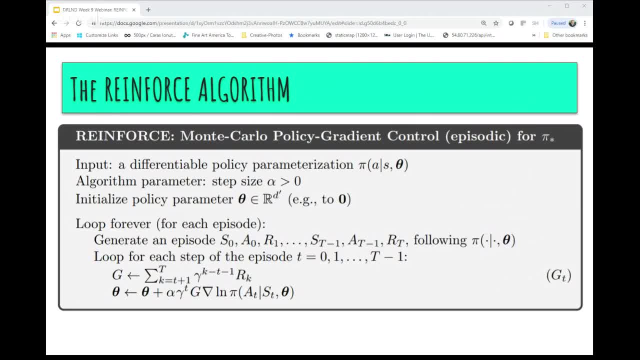 for taking that action in that state and a new state to transition to, and then repeating that until you get to the terminal state. And you do all of those actions following the current policy, which is specified by the current parameters data, the weights. 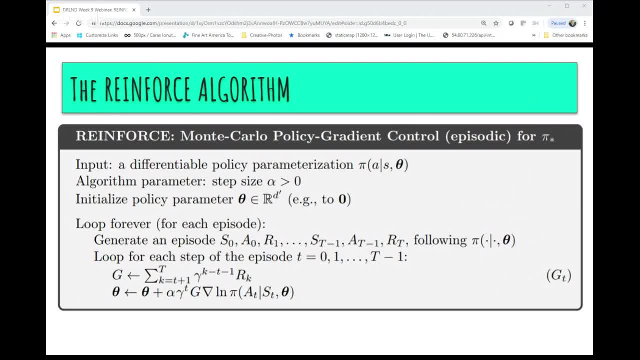 And then you start to analyze how much you've generated. So the first thing we need to do is go through and generate the total return G for this episode. Then, once you've generated that entire episode, then you start analyzing all of the values of 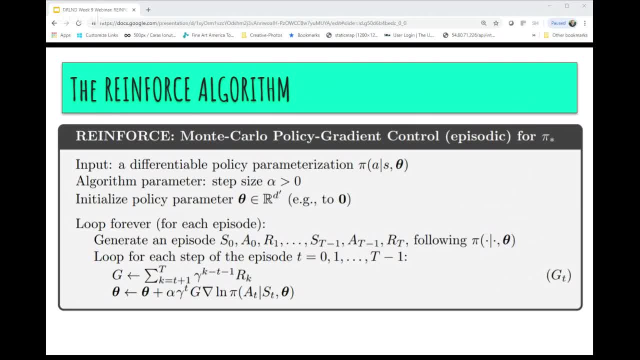 those that episode. First thing that we need to do is go through and generate the total return G for this episode, And we do that. It's a discounted return, So you see a gamma in the formula there and you basically discount each of the rewards. 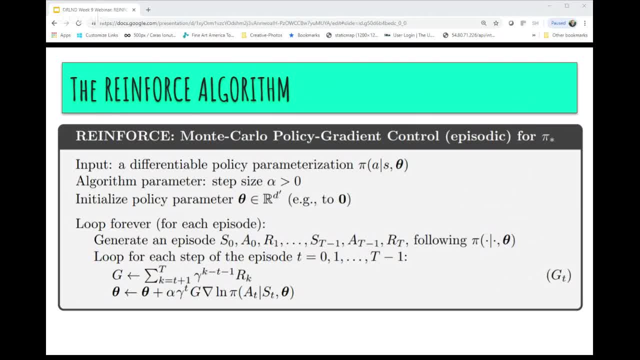 Based on. you know what step they were within the sequence, Got it then. once you determine the total return G, then we can go ahead and make that update to the parameters data, the weights of the neural network, and you basically replace the current values of 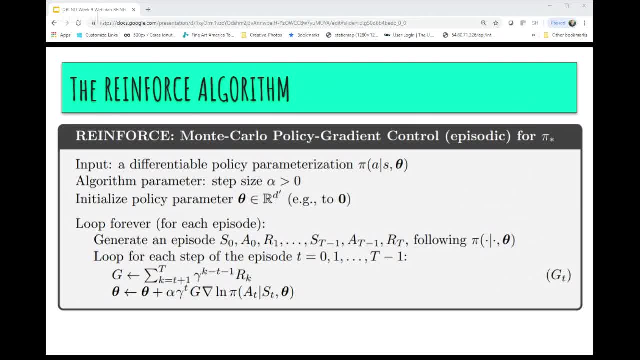 theta with a new theta that starts with the old values, adds in that alpha value times, gamma. now previous slide: we didn't really talk about gamma because it didn't sort of simplify things by not doing a discounted total return. on here we're actually doing a discounted return, so we have 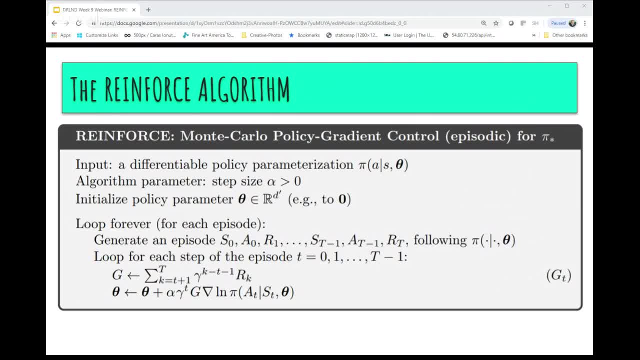 gamma to the T value and again gamma should be a value between zero and one, and so that discounts a future rewards more than the more current instant rewards. multiply that by as a total return that we got G, which we calculated, and step above, and then that's multiplied by. 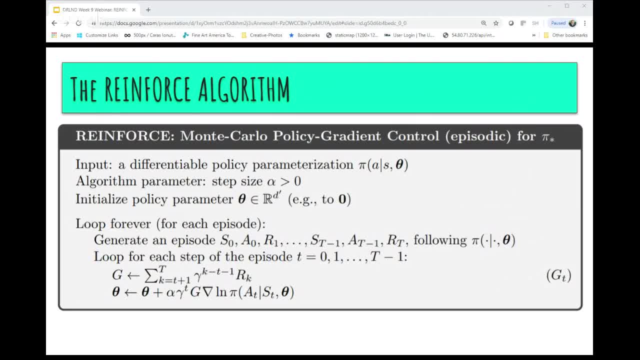 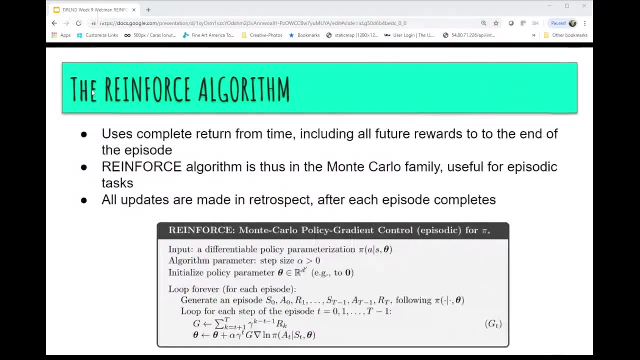 the gradient of the log of the, the policy of actions that you, that you took in a particular state, given that, that, that that value of the current weights of the network data. so pretty simple algorithm. this is repeated here on the slide, but I just want to mention a couple things. remember that. 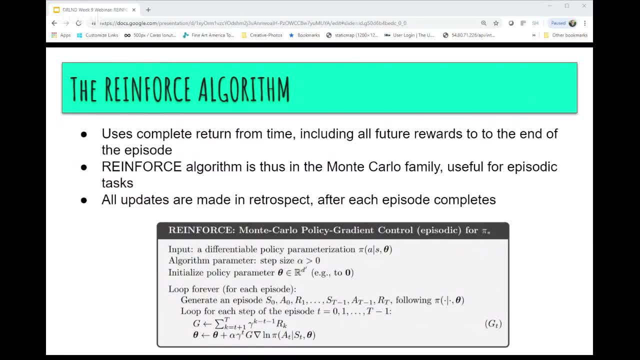 it. it is Monte Carlo, so you can it. it's a complete return from from all time through the entire episode. it's good for episodic kind of tasks- it doesn't work as well- and and tasks that are not episodic And all the updates to the network. 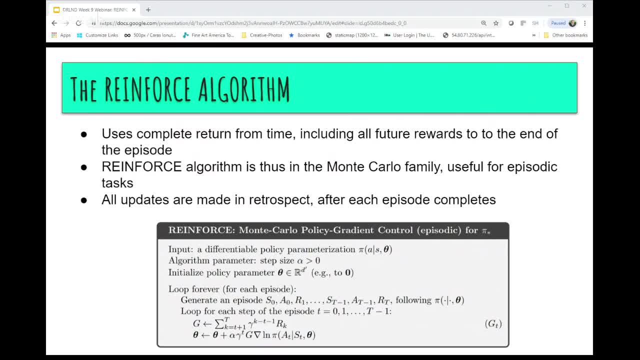 are made in retrospect. You have to wait till the entire episode completes, all the data is available. store all that data into a set of data structures And then, once that's all done, then you can go ahead and make an update of the parameters. 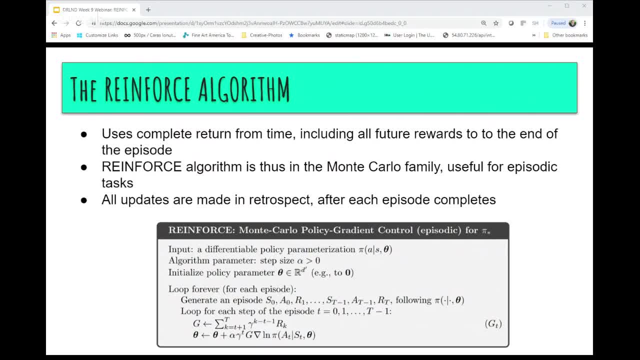 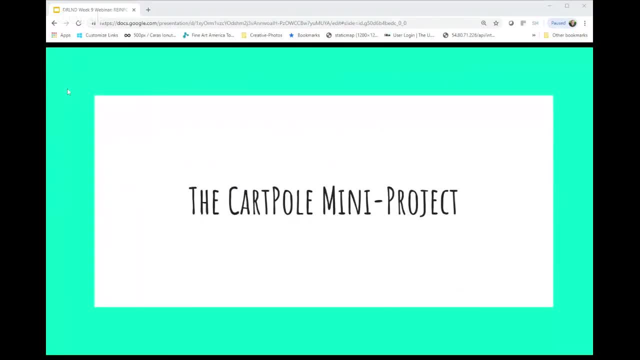 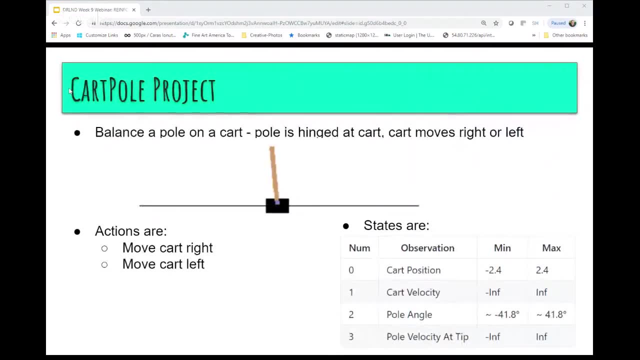 and then repeat the next episode and do the same process over again. OK, so let's apply this reinforced algorithm to the cart-pole menu project. This is a very standard project in all of reinforcement learning- Any algorithm that you might work with a lot of times. 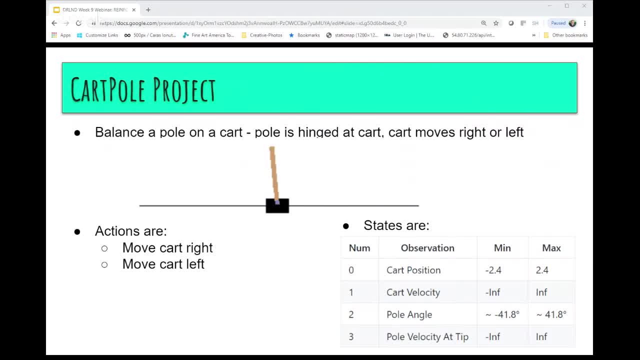 you might first apply it to a cart-pole as sort of a baseline model for how you can compare different algorithms, And it's a very early implementation of reinforcement learning to learn how to balance this pole and a cart. So essentially you've got this pole. 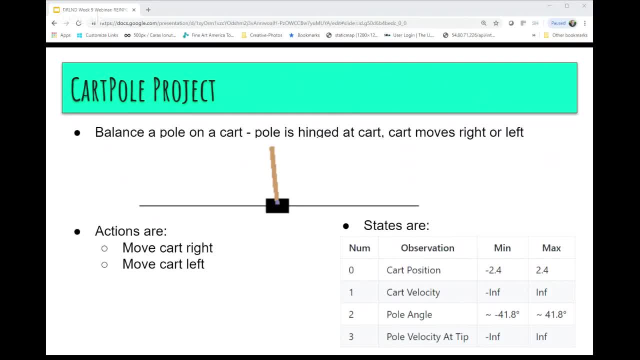 It's got a hinge where it attaches to a cart And you try to balance this pole. You try to have an agent that learns how to balance this pole by taking a couple of different actions, And the only actions available are pushing the cart to the right. 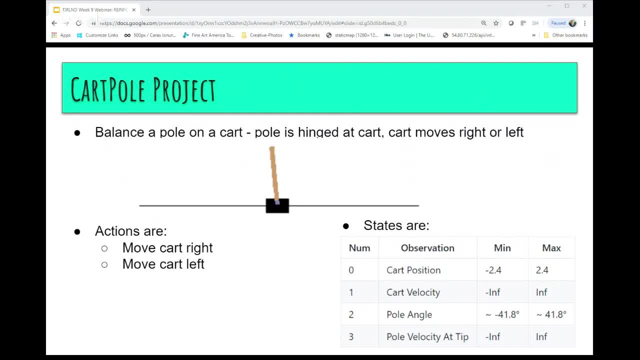 or pushing the cart to the left And, as you can see, if the pole is starting to fall to the left, you would push the cart to the left and it would help balance it, But then, if you overshoot, the pole will start to slide to the right. 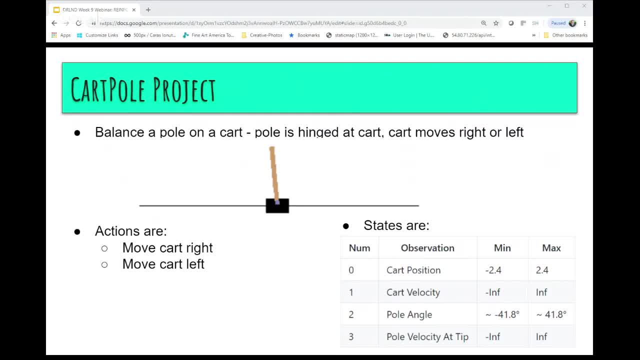 So you need to push the cart back to the right And there's a window that you can't exceed. typically, left and right You could. you know They keep the cart also positioned someplace between those bounds. So the states are very simple. 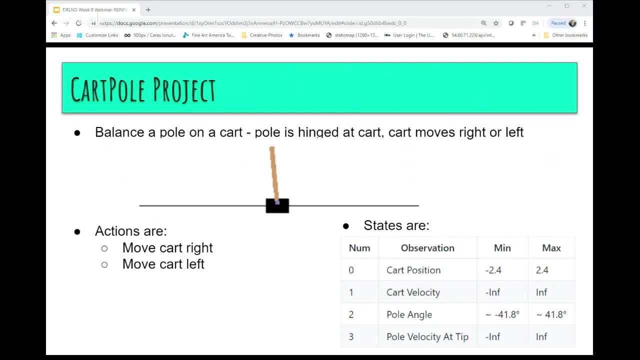 There's a four-state set of values that define the state of this closed system. The first one is just the position of the cart itself and how fast the cart's moving. That includes a direction component. And then the last two are related to the pole itself. 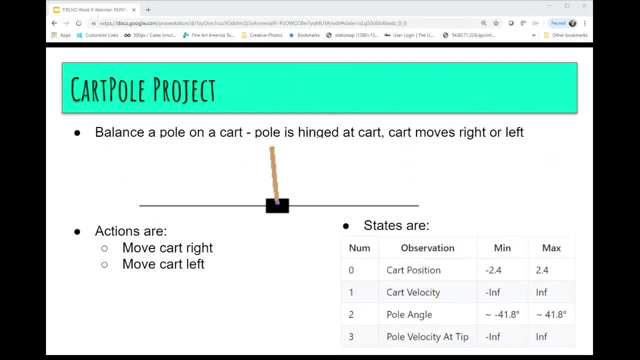 One is the pole angle from the horizontal and then the velocity of the tip. So if the pole is falling fast, the velocity of the tip will be fast. If you've got it pretty well balanced, the velocity of the tip will be near zero. 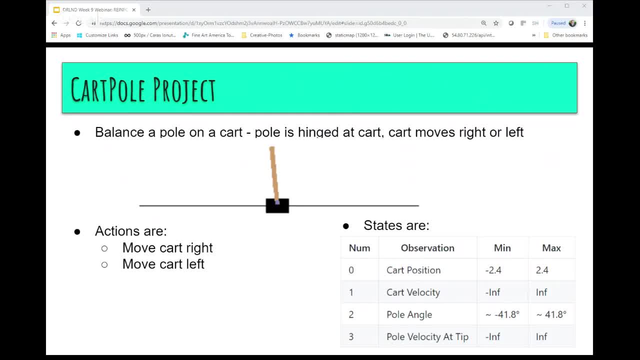 So the goal is really hopefully to have the agent learn how to balance that pole with zero velocity at the tip and make very small adjustments to keep it balanced there. So, given those inputs, we want to input those states and then teach a neural network, a policy. 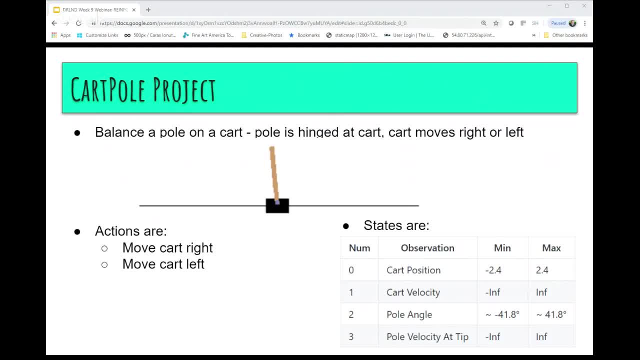 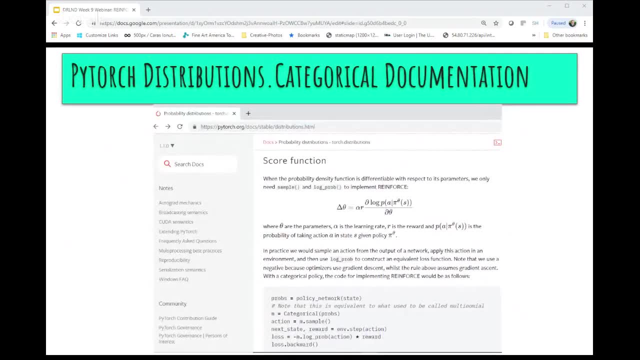 that it can use to select actions based on those inputs. Pretty simple, So I'll mention here. it's worthwhile, when you come across these types of problems, to take a look at some of the documentation on PyTorch. This is a page out of the PyTorch documentation. 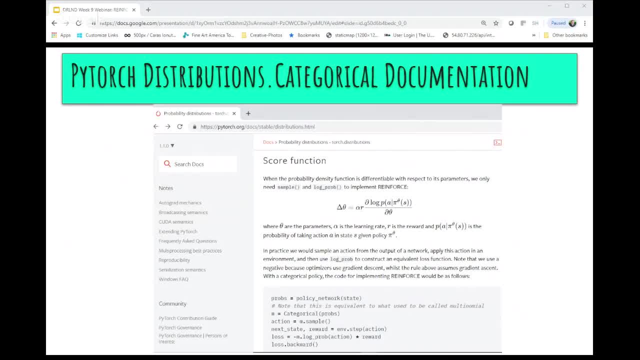 You can see the URL there, One of the things that's used, as we'll see here in a second. I think I included this rep. I didn't include the entire code, but I think I included the reference to a function in PyTorch called distributions. 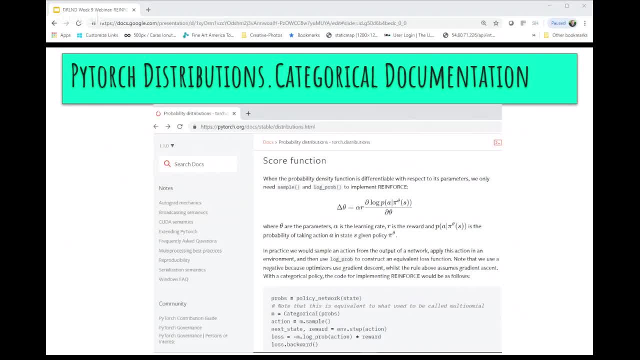 I'm sorry, not a function. a library called distributions And it's got a a family of algorithms within that library. One of them is called categorical, And those categorical functions are very useful And, in fact, when it introduces these categorical functions, 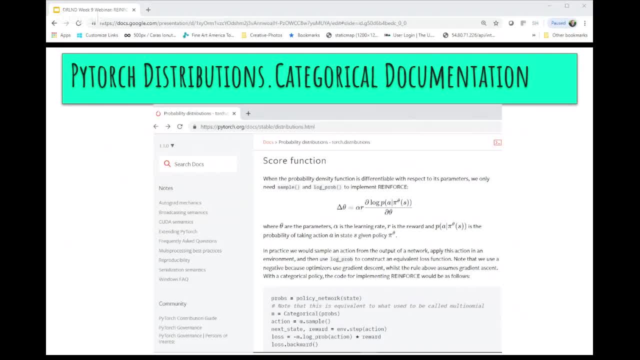 in the PyTorch documentation. it actually uses reinforce as an example And you can see the definition of how this is determined and then a really short five or six line implementation of reinforce And we'll see the version we're going to implement is very similar to this. 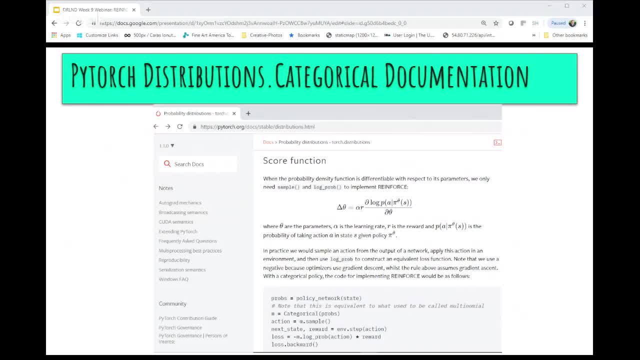 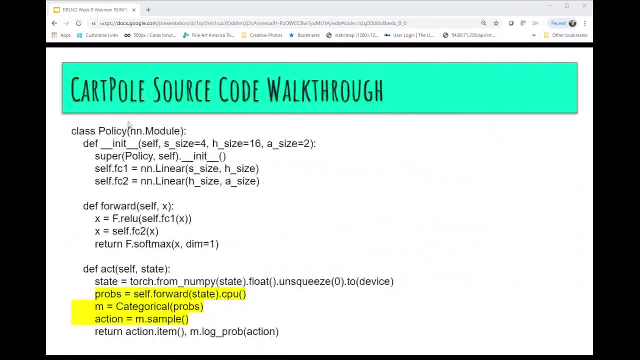 It's a little bit more detailed, But basically it follows the same structure And, again, it's worth reading this documentation when you're trying to learn about these algorithms. that can give some insight into how they work. So let's just do a quick walkthrough of the algorithm. 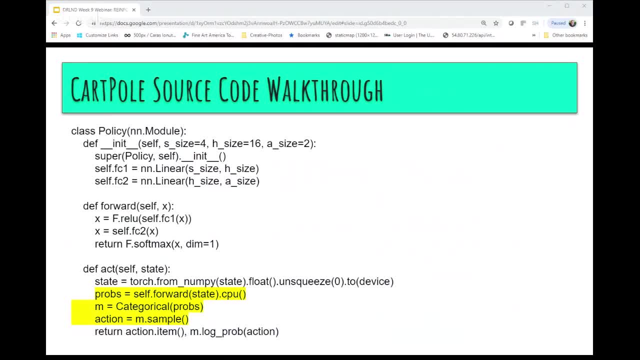 I've got basically two slides here. This first one actually shows the policy class You'll see in. you've already kind of already seen in some of the- probably the first navigation project that you did- Typically the way these algorithms are all implemented. 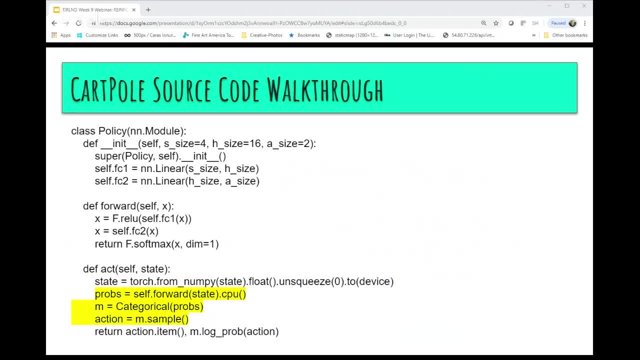 there's two classes that are used, employed, and then a main program or a main Jupyter notebook that instantiates these two classes and actually uses them to implement an algorithm, And those two classes typically are a model class that would define. 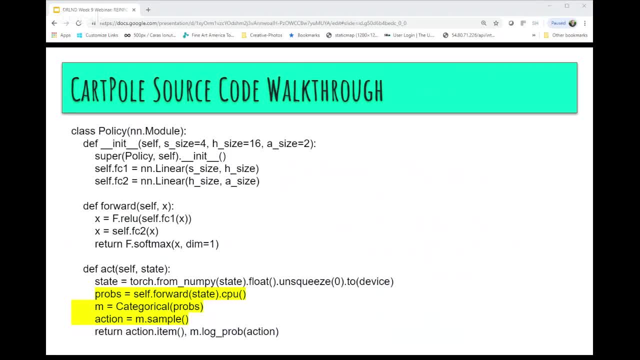 the neural network model And that's what this policy library that you see here, this policy class is. And the second one is usually an agent class that actually implements the agent code. But here let's take a look at if policy as an example of a neural network model. 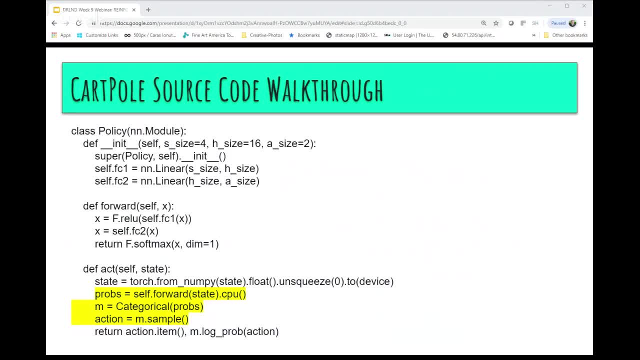 It's a very simple model, as you can see. It has an input layer. As we saw, there's four. there's four values that make up that state. The value value is the same value. So if we apply the five values, 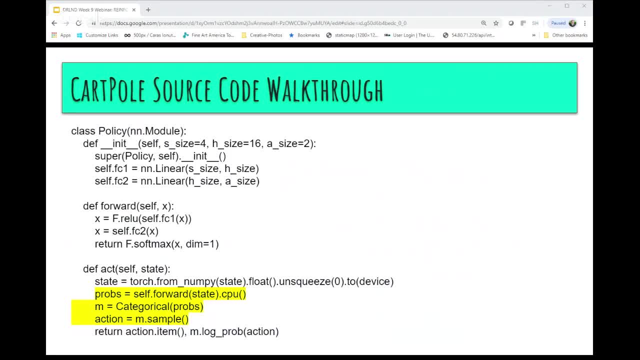 state the values we talked about earlier, with the position of the cart, the velocity of the cart, the angle of the pole and the velocity of the tip of the pole. so those are the, the input states, and your only two actions to choose from are move left and right. so the inputs. 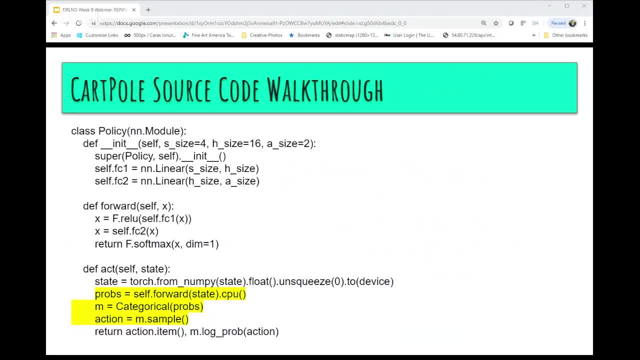 are those force neurons and then the outputs of those two neurons that define the uh, the actions to take. and in between is a simple uh, very small uh, 16 node, uh hidden layer. you know it's very, very simple uh network. as you can see, the forward uh step uh just basically uh inputs the uh, the states. 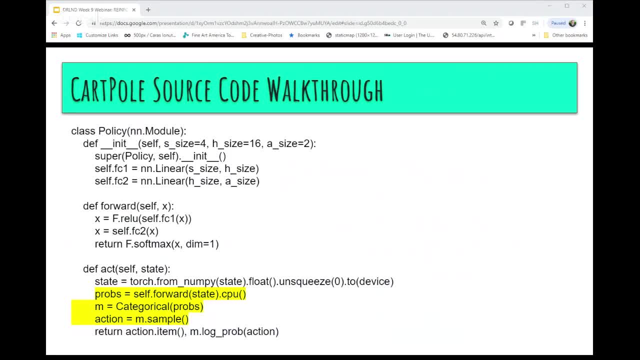 uh performs a uh, a fully connected uh um layer to the uh, to the hidden layer, and then uh does a simple radio activation function and then outputs uh the value from that as a softmax function. so again, if you remember from your no network class, the softmax basically tells you a probability of which of uh distribution for the actions. 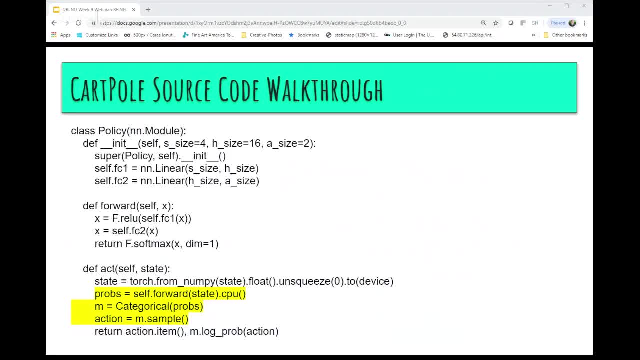 the outputs, in this case, which are our actions and uh, those probabilities will add up to one. um, so if, if, uh, stochastically, uh, you know the, the actions are equally probable, they would both be 0.5. if, uh, you know one of them is 90 percent, uh, more likely to. 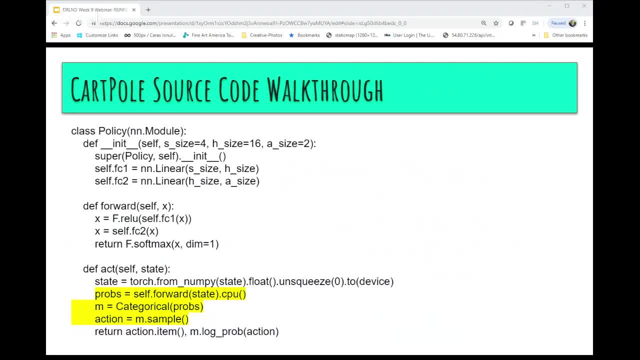 uh should be picked, then it'll be a 0.9, while the other action will be 0.1. it'll always add up to one and then uh the act function. uh, act function usually is actually uh implemented in a in an agent class. uh, in this particular implementation of reinforce, they didn't uh include an agent class. 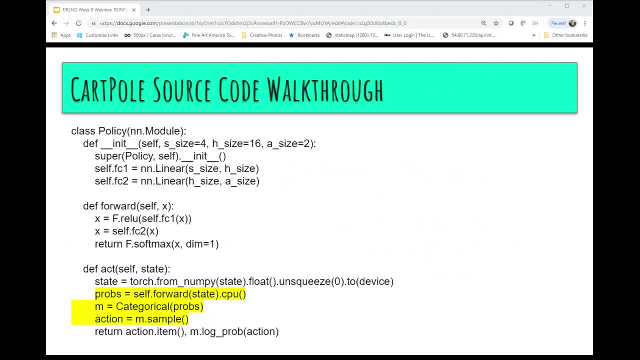 so, uh, they've included this act uh function as part of the policy. uh, essentially, it inputs the state uh taking those, uh those values uh that were just input as, uh as a numpy array converts them into a, uh, a pie torch tensor. that's what the first line does. 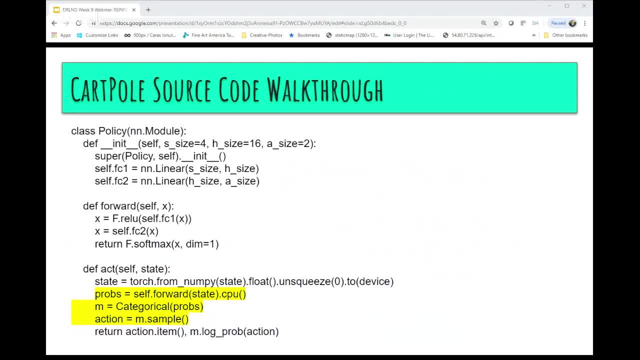 and then it calculates the probabilities by doing just a forward pass through the network. and then, uh, this categorical- uh, that's the function i was telling you about as part of the distributions package in pytorch m- is a categorical class until you define that based on the probabilities that you got, and then the action is just a sample from that class. 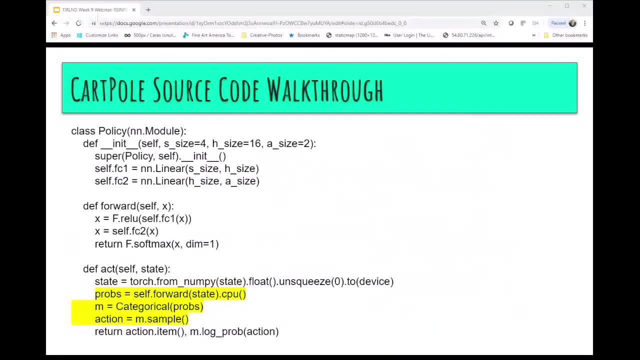 and, uh, it samples from that class based on those probabilities, uh, so that, uh, you know, actions that have a ninety percent chance of probability would be picked ninety percent of the time. those with, uh, you know, 0.1, we would be picked ten percent of the time. and then, uh, the function. 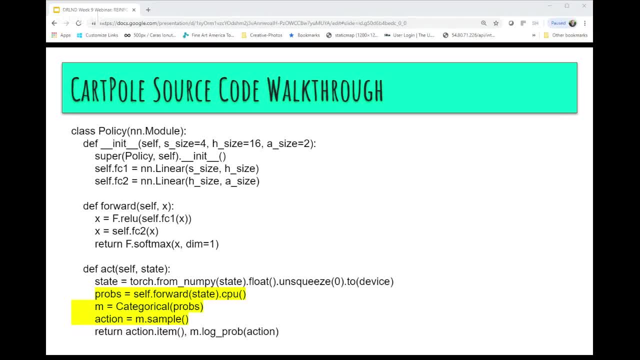 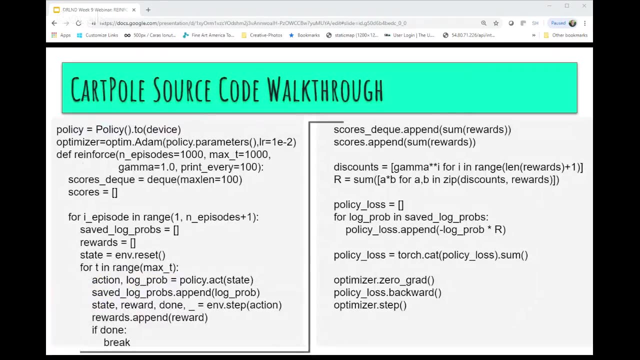 uh act just returns the selected action uh, along with that log probability value for the action, and that log probability is going to be used as part of the uh, the training. so that was the policy network, that's the neural network part of this algorithm. the next part is the actual. 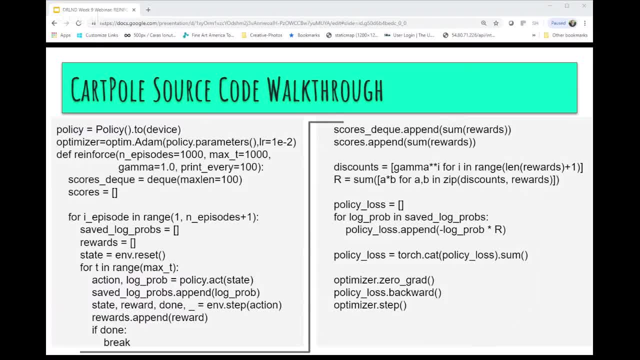 implementation of reinforce. um, you can see the very first line and again, this is uh, not the entire algorithm, it's a snapshot of the middle of the algorithm. i kind of pulled out the most important parts here at the top you can see we instantiate, uh, one of those neural networks and we just call. 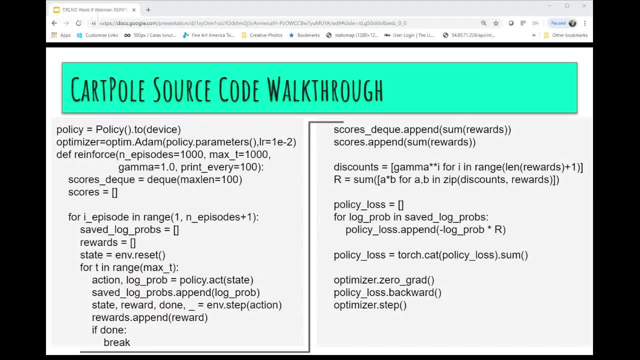 it policy. we set up an optimizer, in this case an atom optimizer. it's a very commonly used optimizer for training neural networks- and then we define the reinforcement algorithm, with the number of episodes that we want to run through and the max number of mini steps within an episode, the gamma. 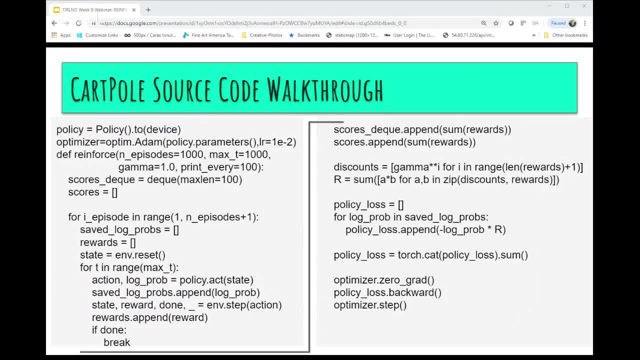 factor, and then define a couple of variables here for storing some intermediate data, a deck of scores and the actual list of scores, and then we go through this loop and this loop basically loops over all the episodes. so, since we defined the default, if you call this with the default of a 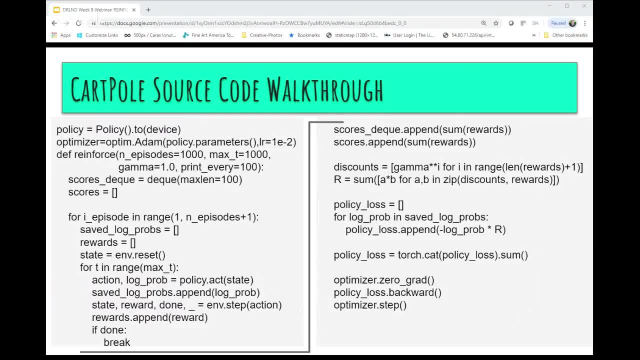 thousand episodes. it would go through this loop a thousand times and it, you know, initializes some variables for the saved values of those log probabilities that we just saw come back from the act function. it initializes a set of rewards. these are the rewards for every step of the episode, so we'll 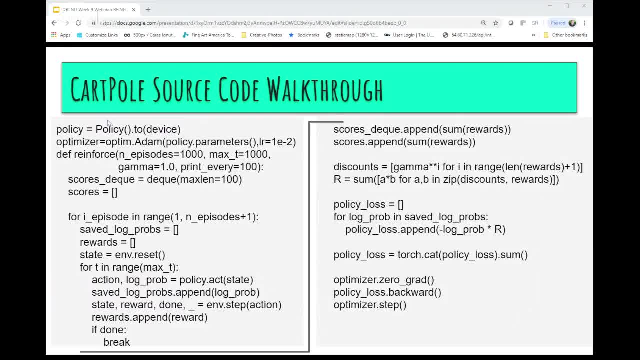 be saving all those and remember, since this is monte carlo, we have to save every episode from each, each state transition. so each step of the episode, we need to know what those rewards were, and then this state, basically, is just telling the environment to reset back to the beginning. 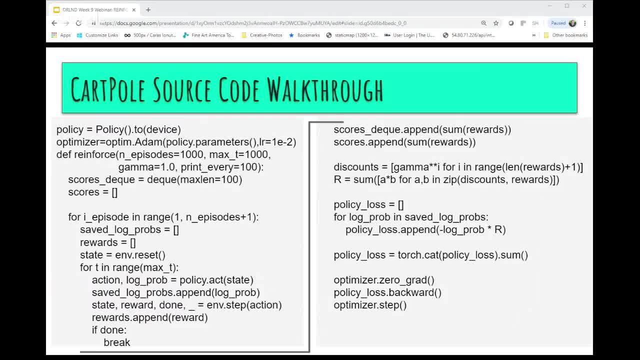 for a new episode, then, uh, we go through a second inner loop of the max t. if this entire length of episode, everyone we wrap this up, atty to decor вообще, can put a bunch of stuff, 4 apps in to any of all. the Chef for the. 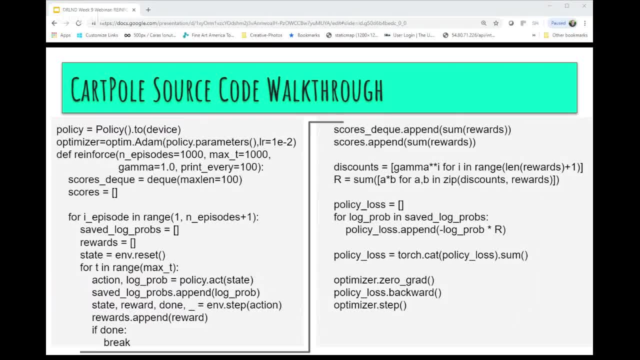 rest of the family, our workaholic. uh, some of this. this change structure as well as selected and we're certainly going environment. take a step using that action that was determined from the policy. So it takes a step to the next state and returns to us the next state and the 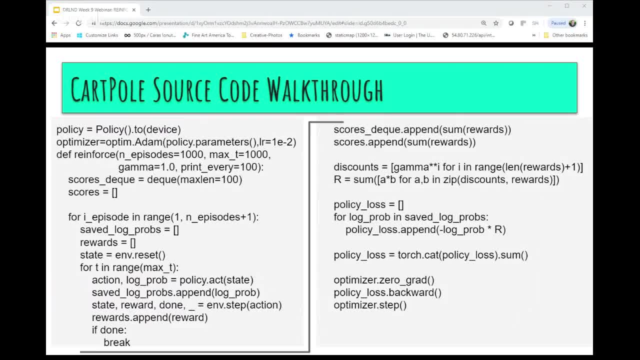 new reward for that transition, And so we save that reward away. If we ever get a done flag, which means we got to the terminal state, then we are done with this inner loop And we keep going through that. either. the maximum number of mini steps. 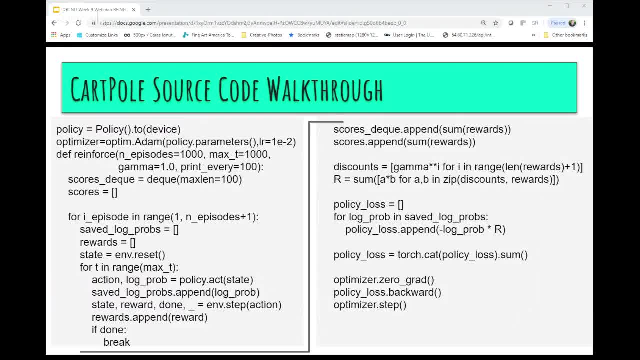 in this case a thousand, or we get to the terminal state And that defines the end of the episode. So once the episode is over, we have all that data collected up, with the rewards we've achieved, the log probabilities, the actions that were taken. 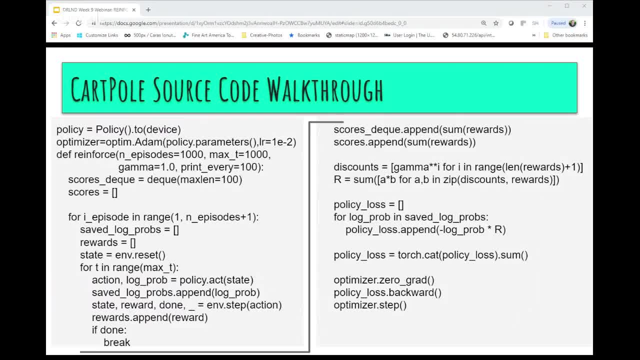 all that information is available to us in those data structures. So we start here to implement the inner part of reinforce. We append the total value of all the rewards that we've got to the scores And likewise to the scores deck and also to the total scores list. 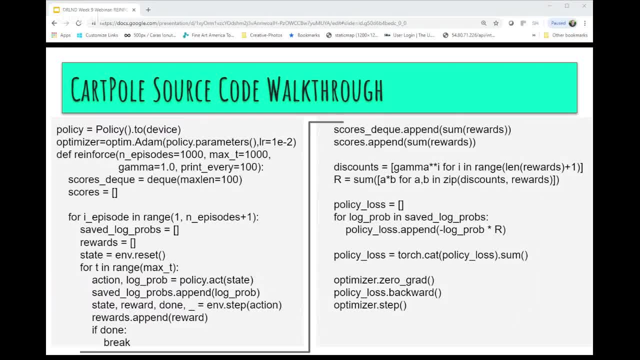 And then we calculate the discount factors, which is basically the discount. This is an array of all the gammas raised to the power of I to get the discount rate for every step of the episode And then calculate the total return, which is basically the sum of all the discounted rewards. 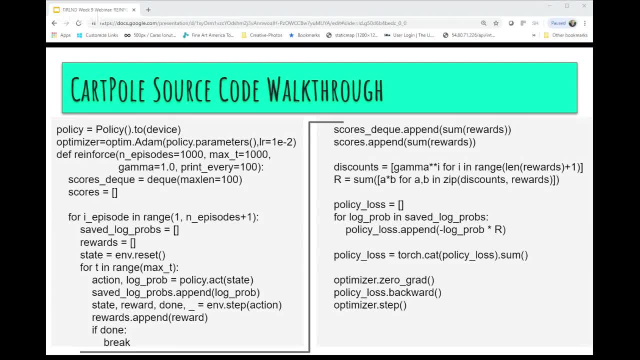 And that just that little Python, A times B for AB and zip of discounts and rewards that basically runs through that entire set of lists of discounts and rewards. applies that A times B to discount each of those rewards to actually get you a total reward R. So now we go into the part where we're going to start getting ready to 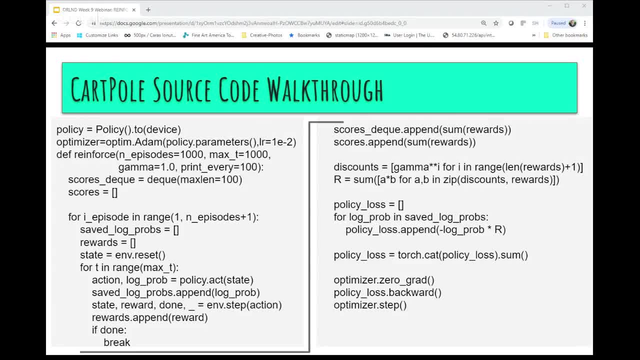 calculate the learning step for the policy network. So we first go through all the log probabilities and append those to the to the policy loss List. in that policy lot loss list then is is used as part of the trainings We'll see here in a second. we first zero out the gradients of the optimizer. 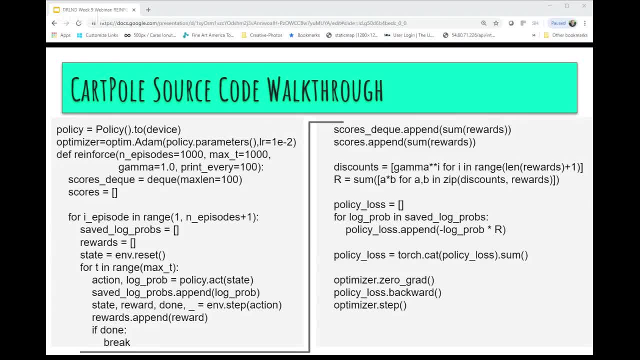 So we start with no gradients. We do a backward propagation step, which then propagates all the errors back through the network and uses that policy step as the optimizer to actually perform the propagation. That represents one step of learning. once that the weights were all been, 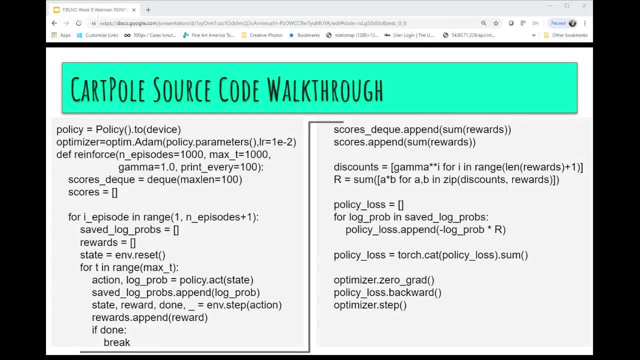 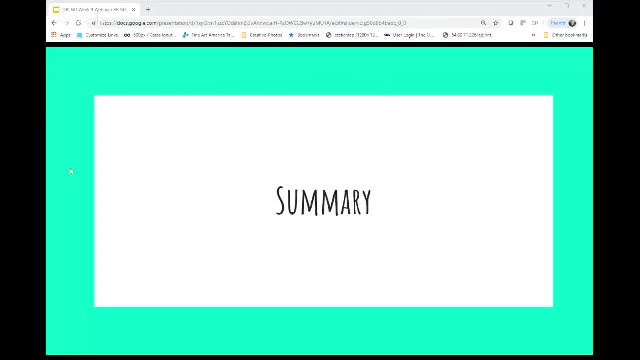 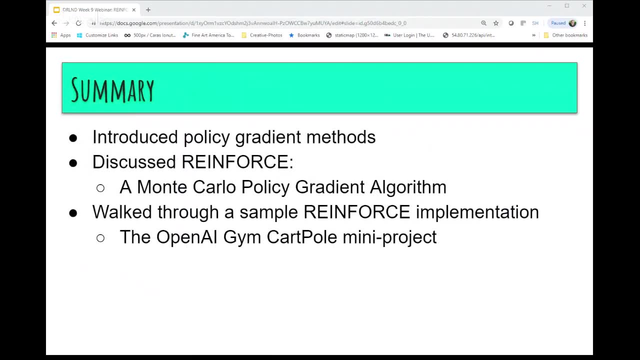 adjusted. we go back through and do the next episode. so that's all repeated. you know as many times as you as you have episodes. so fairly simple process. I we should mention there's a mini project in the in the course. it has a notebook already programmed for. you should go into that carpool project and actually I 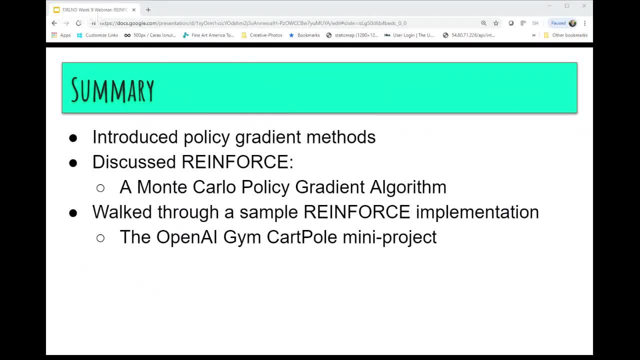 think it's a pretty good idea to execute each the cells in that notebook and watch the network get trained and then watch it actually perform the the with the environment, learn how to solve that environment. and watch, watch it, watch the agent, the trained agent. when you're done actually move the cart to keep that pull. 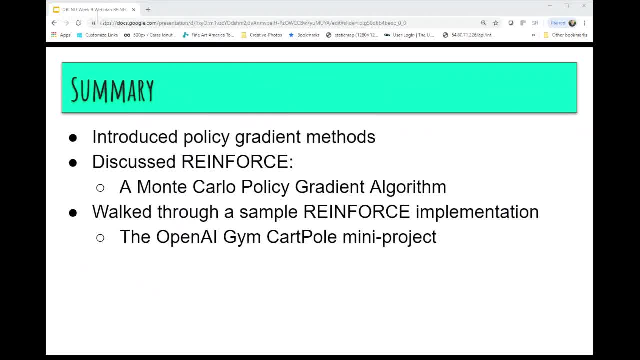 balanced. it's a very simple four or five different cells, most of them I've already talked about here. just execute each one of them and it doesn't take very long, Maybe a minute or less. It's actually train. that network is very efficient. takes a few hundred episodes. 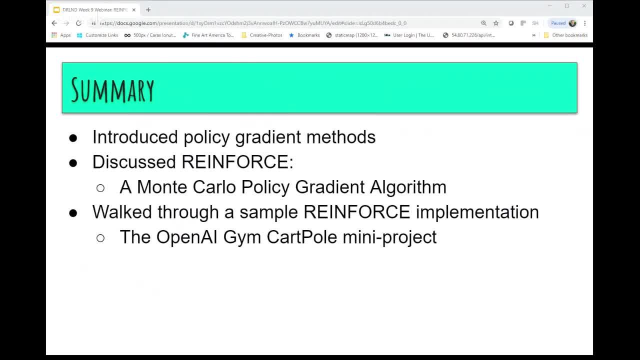 and and and it's. it comes up with a policy that can can balance that, that poll. so pretty impressive. so, in summary, this evening we discussed, introduced really policy gradients- this is the first introduction of policy gradients- and we talked about how policy gradients, the theory behind them, how they work and 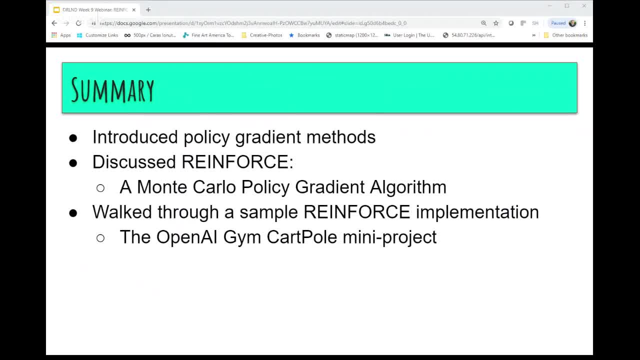 then we applied them in this reinforced algorithm, which again is a Monte Carlo policy gradient algorithm, so requires us to actually, you know, go through the entire episode before we can make updates to the policy, and then we walk through an implementation to reinforce in the open. IGM carpool. 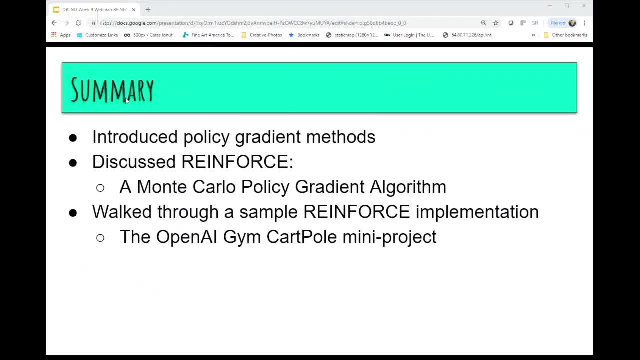 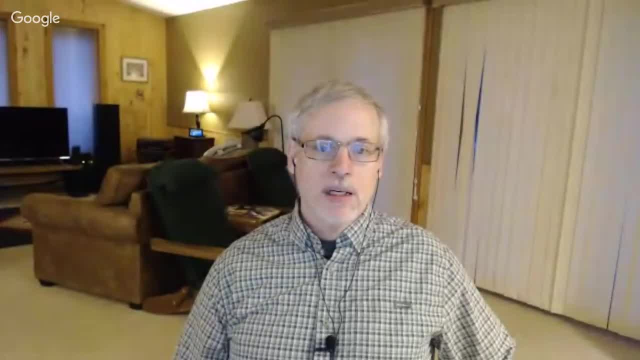 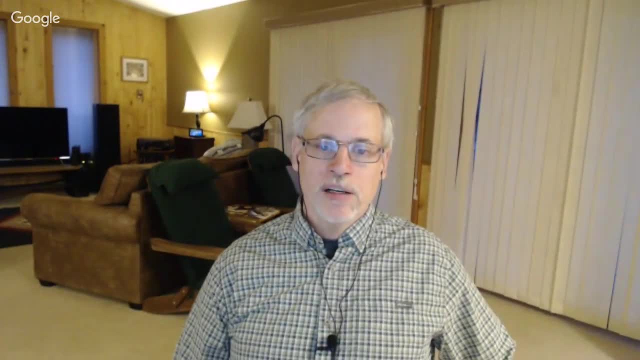 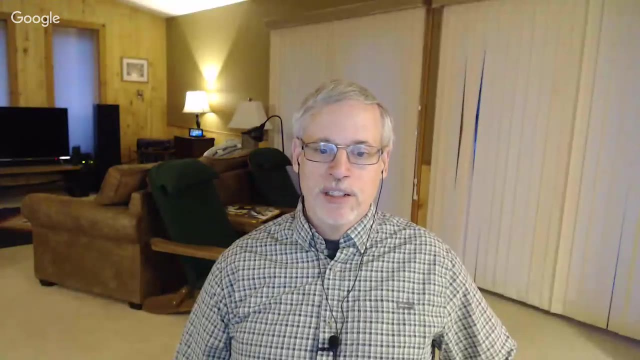 project. so with that, if anyone has any questions about tonight's topic- I have asked me anything. session immediately following here it's on slack, so if you like to tune in there, ask any questions, be happy to answer them live. and with that, that is tonight's webinar and we'll see you next week. bye.